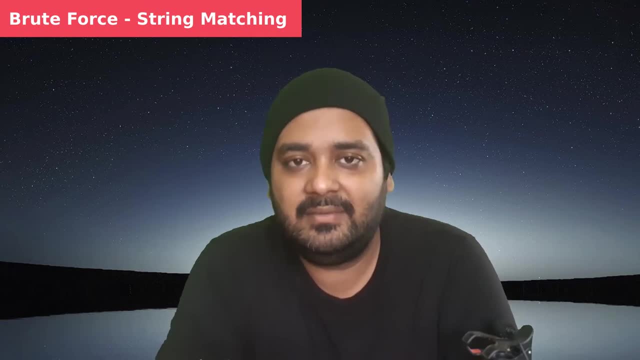 just do it operation to solve your problem. so, which means that if you're having n number of solutions for the problem, it just tries out all the solutions to find out the optimal solution for your problem. so this is how your brute force algorithm works. so here we just shall look at how 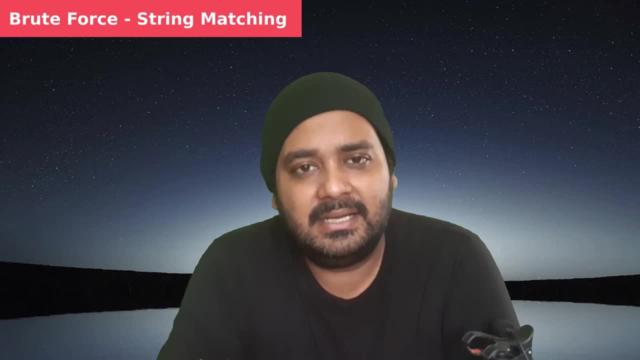 our string matching works. okay. so let us take a particular string, given string. okay, so string is nothing but a sequence of characters. we just know it and you will be given with a pattern, okay, so what we have to identify here is whether the given pattern is available inside the given. 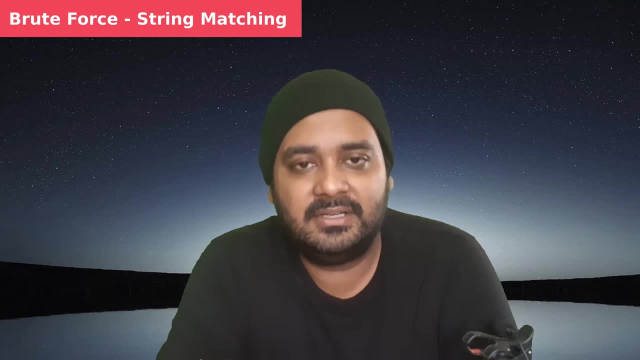 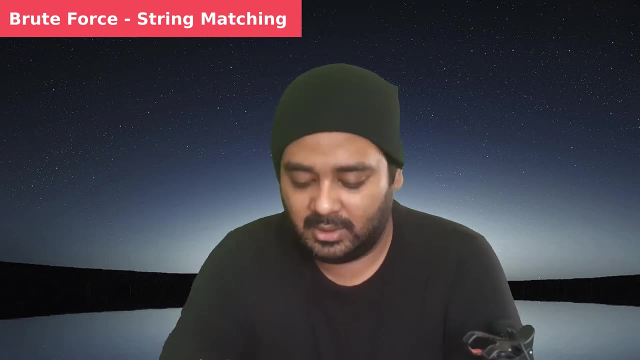 string or not. so, for example, i just want to search a number of term, not means, whether it is present inside the particular uh thing or not. i just have to mention it out, okay, so what we shall do is that we just shall look at it with the help of an example right now. okay, so this is the given. 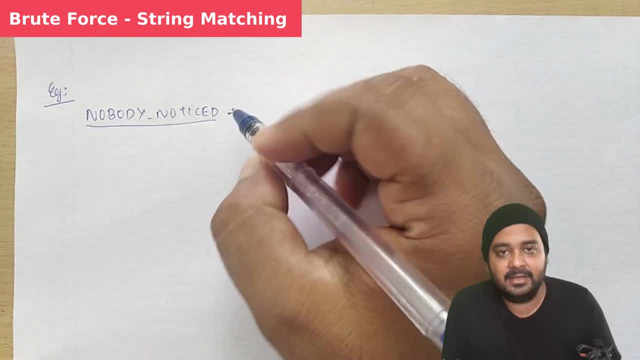 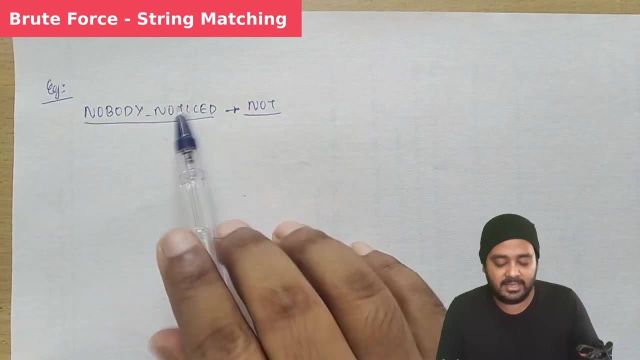 string. so, uh, what i have to do is that i just have to find a new element out of it. so the new element which i'm just going to search is not so, which means i just want to search the the presence of not inside this particular string. okay, so what is this first step i have to do is 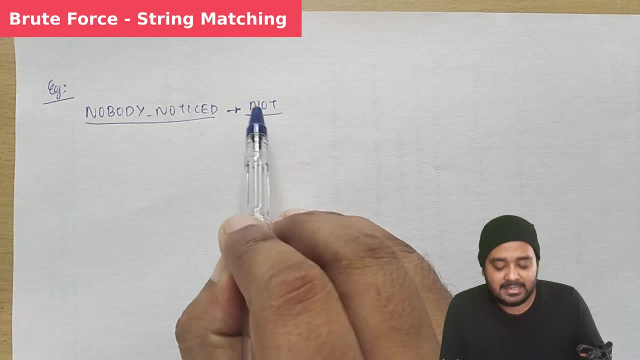 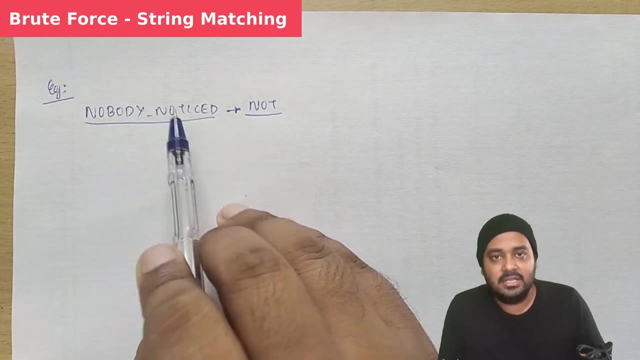 that i just have to take the first element, which is nothing but, uh, inside the search key, okay, and i just have to compare it with the first element inside the given string. so if it matches, i just move on with the next. so, likewise, i just keep on moving right. so the incremental process will. 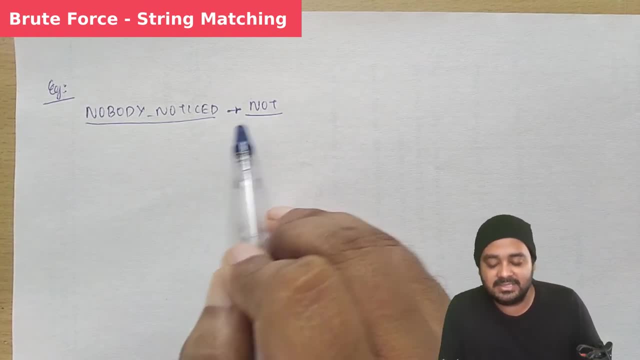 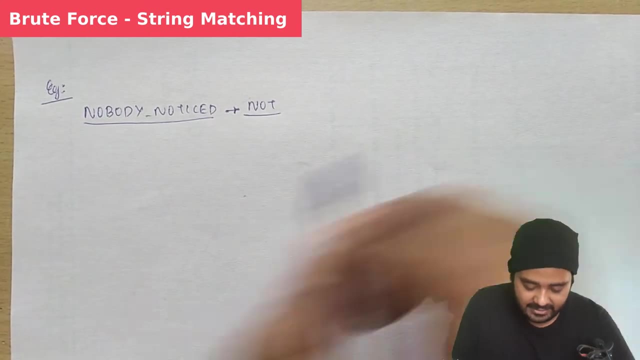 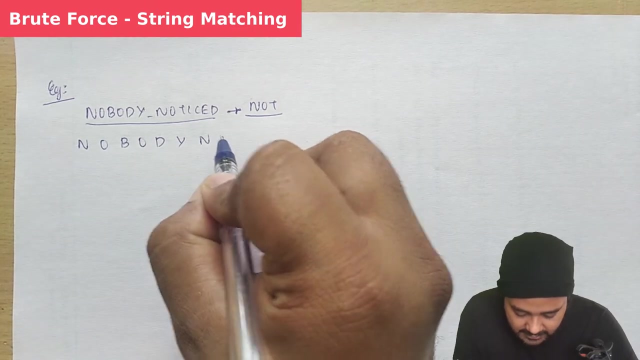 continue inside it one and only if the particular string matches. if it doesn't match, the entire first string will move on to the next string. so, for example, i'll just mention it out right now: right, so the same example. so n o, v, o, d, y, n o t, i, c, e, d. right, so this is the 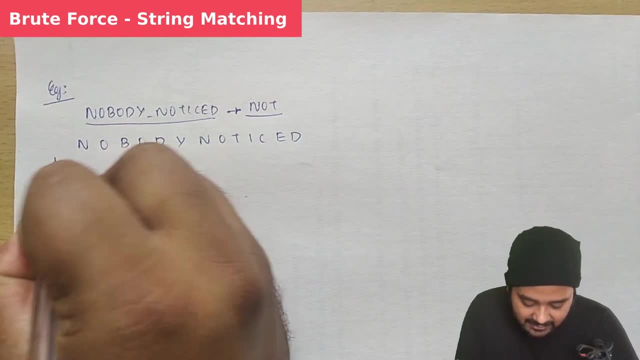 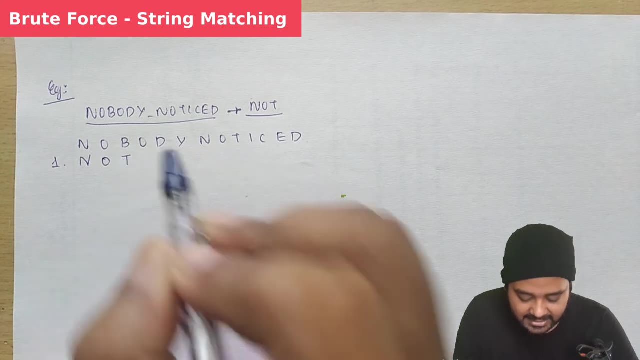 given string. so what i have to do is i just have to check it with it. so the first step, what i will be doing, is i will be taking the first element n right so, from the given search key. so i just shall write out the search key again. okay, so what it does is that it just checks whether this 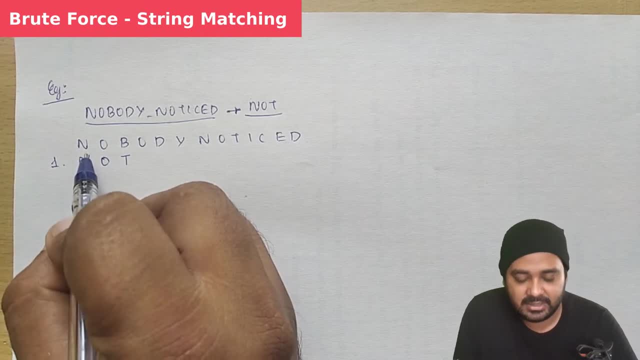 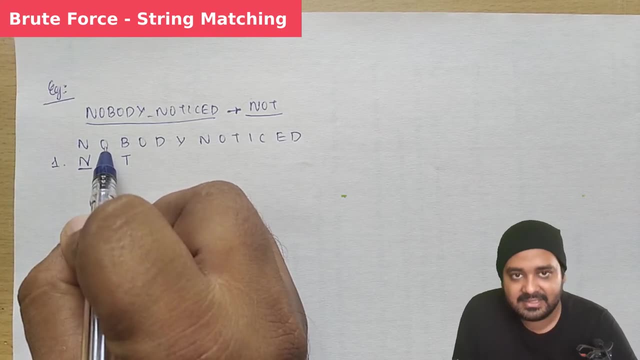 particular element matches, so these two elements match. so what it does is that once, if the particular element matches, it just moves on to the second element inside the string and then compares it with the given string. okay, so, search key, it just takes the second element and then compares it with the given string. second, 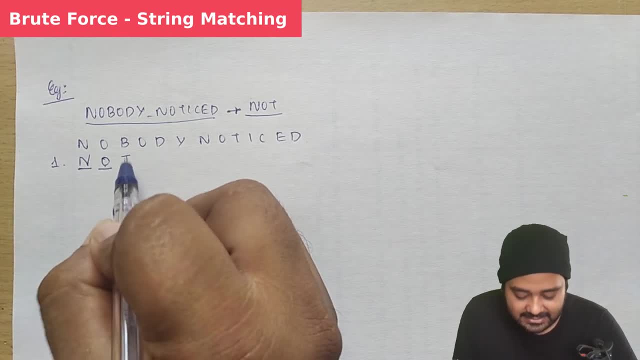 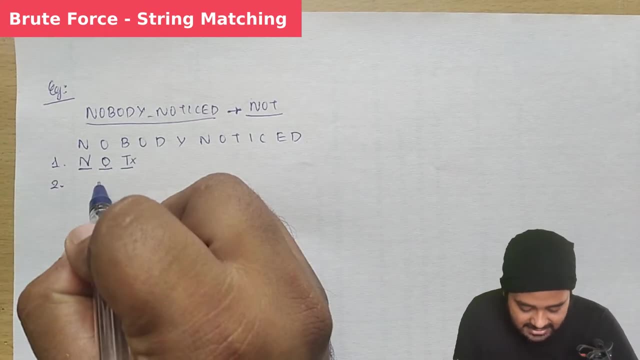 element it matches. so what it does is it just takes the next element and just compares. so here it is not matched. so what it will do is that it will just move on to the next iteration. so next iteration also, it just comes in the same manner. so it just takes n o t right, so n o t is matched. 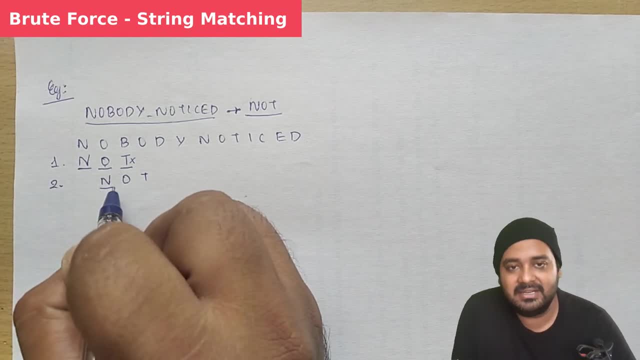 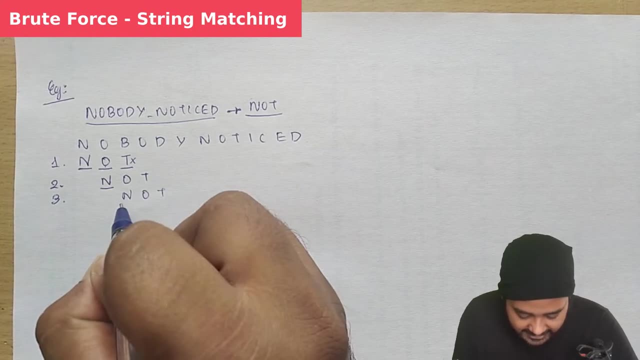 with the given element it is not matched. so whenever the first element is not matched, what it does? it just moves on to the next iteration. so next iteration: i just come up with n o t. so again here, my n is not matched with my b, so i just move. 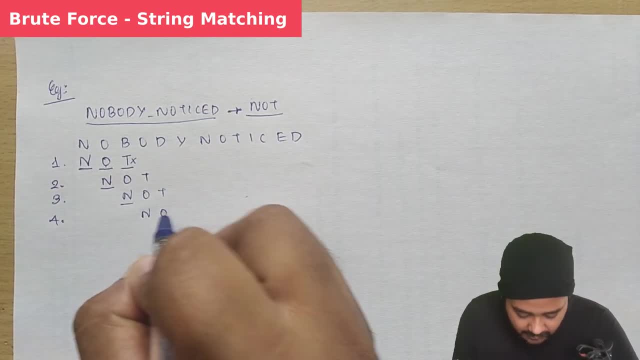 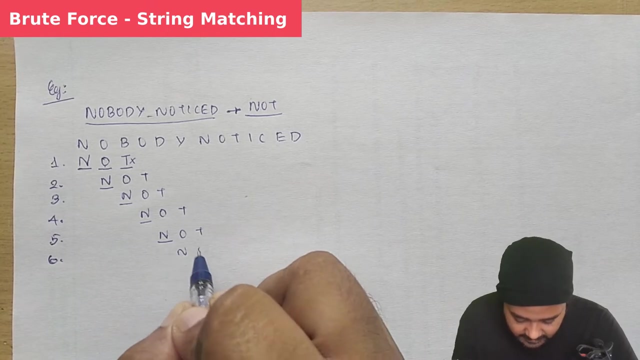 on to my next iteration, which is nothing but my 4. so again what i do: i just compare it, so n is not matched with o. right, so next one. i just compare it again: n o t, so again it is not matched. so i move on to the next iteration. so similarly n o t, so here it is not matched. if it is not matched, 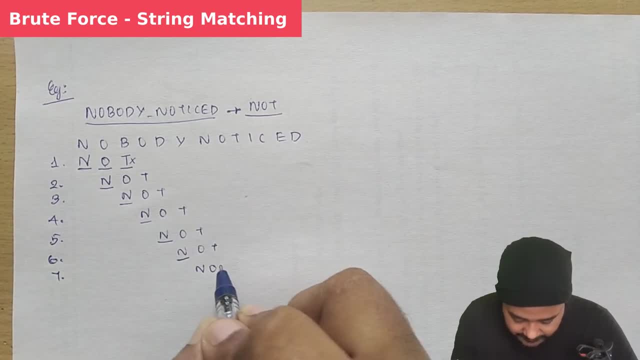 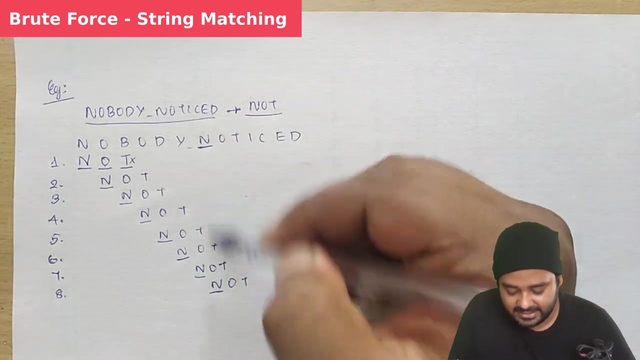 with y, right. so the next iteration. so i just move on to n o t. so it is not matched with the empty space which is given. so it is not matched. okay, the eighth iteration. what happens is that it just matches the element. so here your n and this n is matched. okay, so here, whenever the string is: 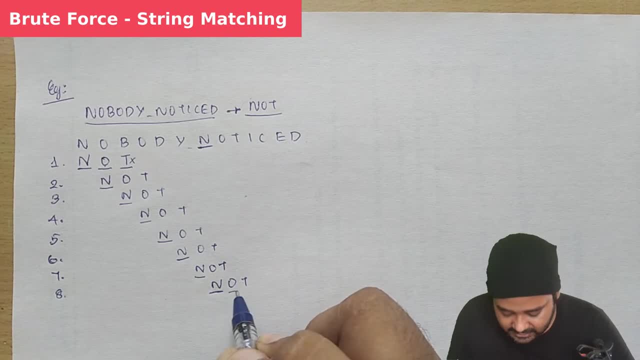 matched. what we have to do, we just have to go for the next element inside it. so now, what i do is i just go for the next element inside it. so now what i do is i just go for the next element, is that i just take the o right now and i just compare it with this o. it matched right, so once. 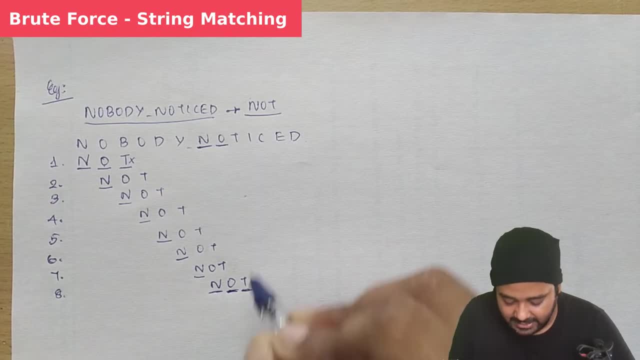 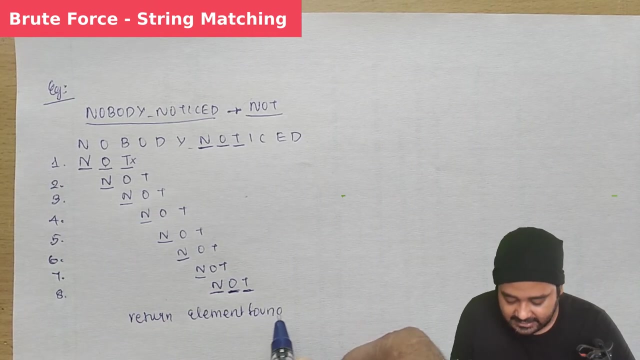 it matched, i have to move on to the next element, so t. so i just take my t and i just compare it with my t over here. so this t and this t is being matched right now. so whenever it is matched, i just return. so what i will do is that i just return element found or i just write it as a return. 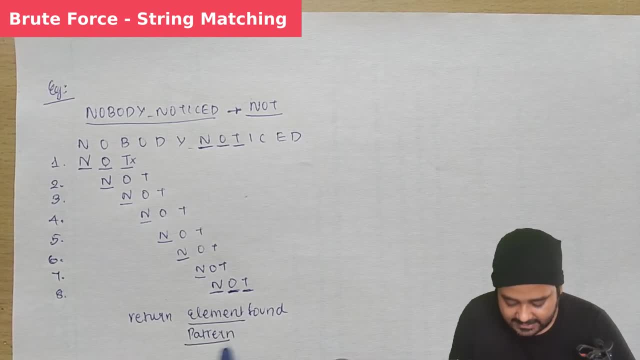 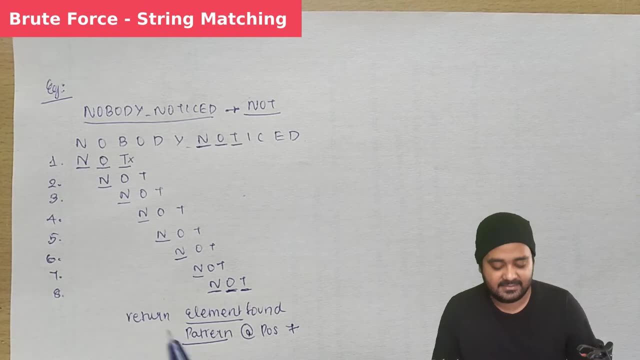 element or pattern. so i just write it as pattern found. so i just write it as pattern found at position seven. so, which means that eighth iteration means we just start with the position zero. so at position seven we just have found out the element, not so. this is how our brute force approach solves the string matching problem. 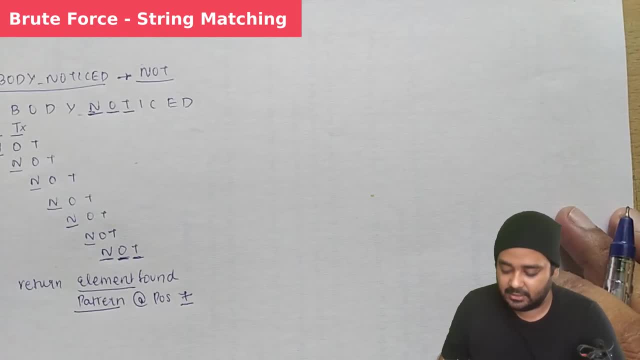 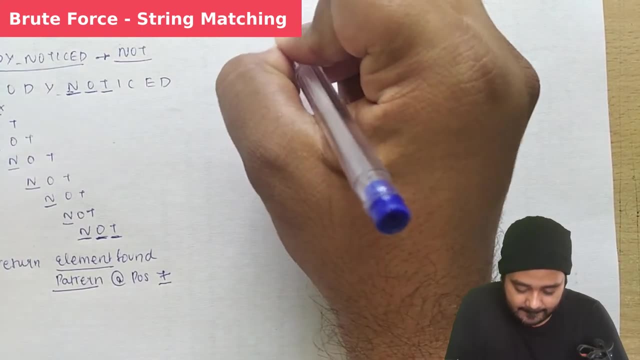 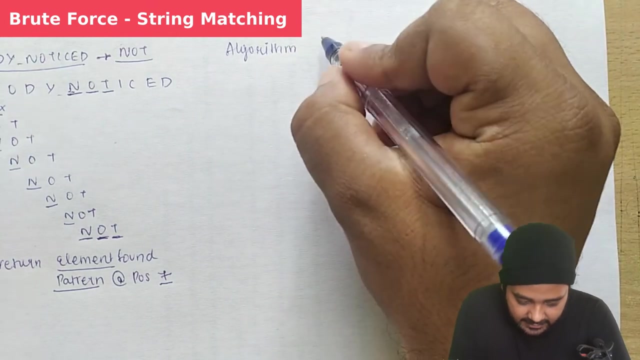 right, so what we shall do is that we just shall look at the algorithmic part of it. okay, so i'll just write down the algorithm. okay, so algorithm always begins with the algorithm. okay, so we just write down the algorithm, keyword, algorithm. right so algorithm, i'm just writing it down. okay, so it is an algorithm for. 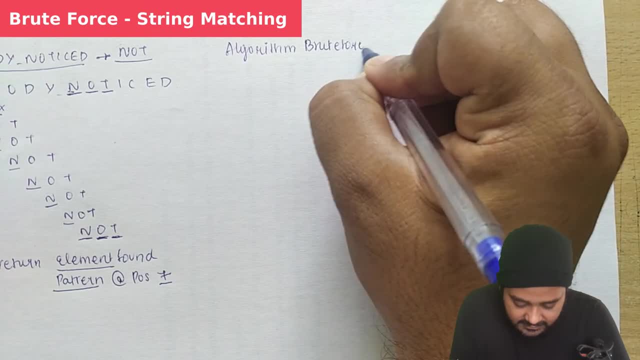 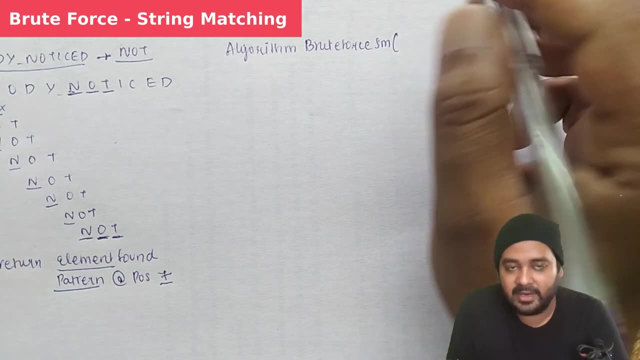 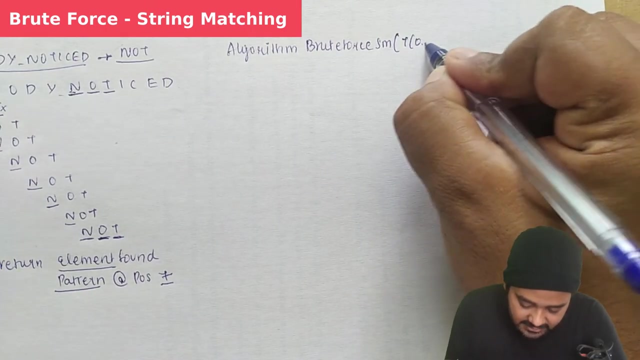 brute force, brute force string matching. so i just uh counted, okay. so again, uh, we are going to give uh two kind of strings, right, so strings will be generally uh passed as a form of a character array. so what i do is that i just mention it out. so zero to n. so this is the first text which i want. 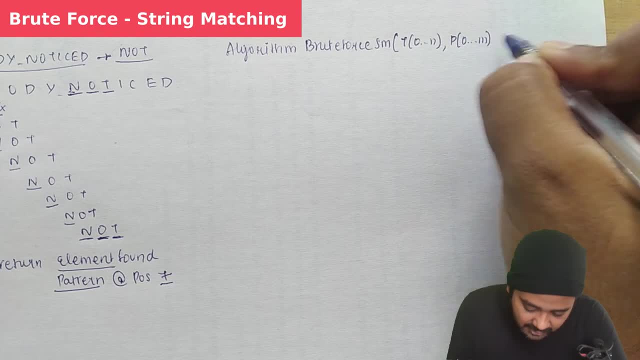 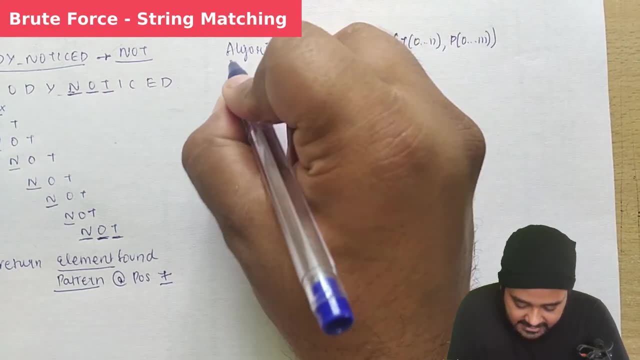 to identify. and then, uh, the next one is the pattern which i want to identify. so i'm just giving it as such. so this is the argument. i'm just passing it as an argument, i'm just giving it as an input. okay, so initially i just have to mention the description. so it is, uh, brute force. 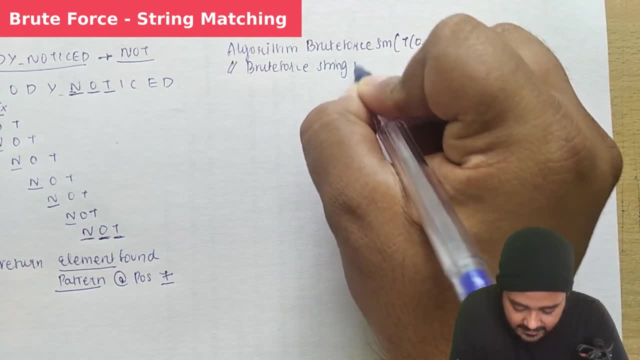 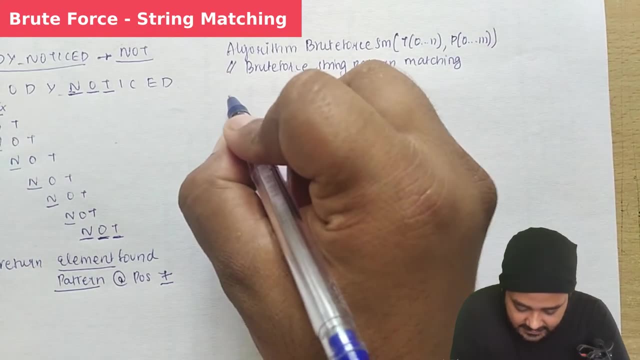 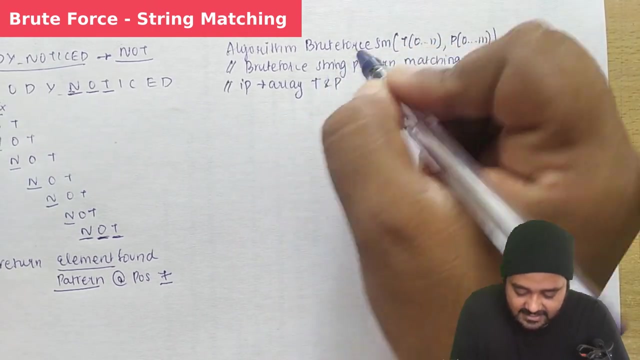 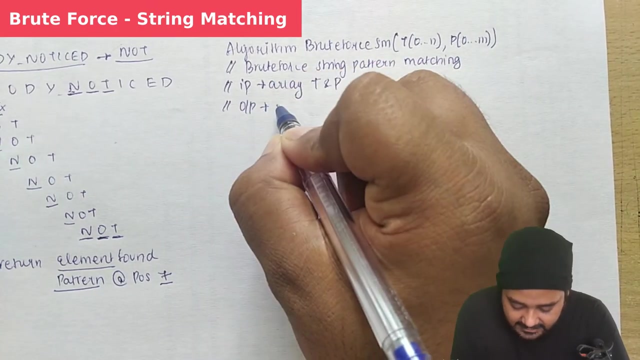 string pattern matching. okay. so it is a brute force string pattern matching, right. so my inputs i'm just going to give array. so i'm just going to give two array in a form of t and p. so t is represents your text and p represents your pattern, right? so again, uh, my output will be in a form of either uh element position. 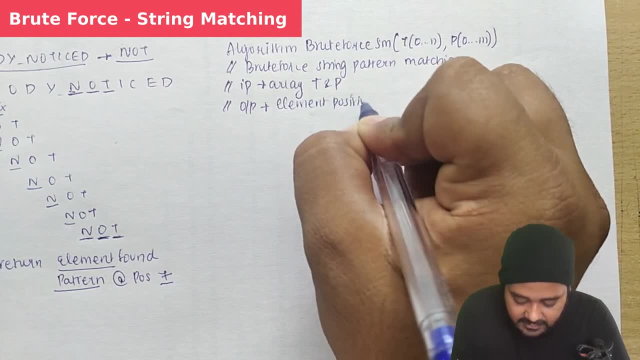 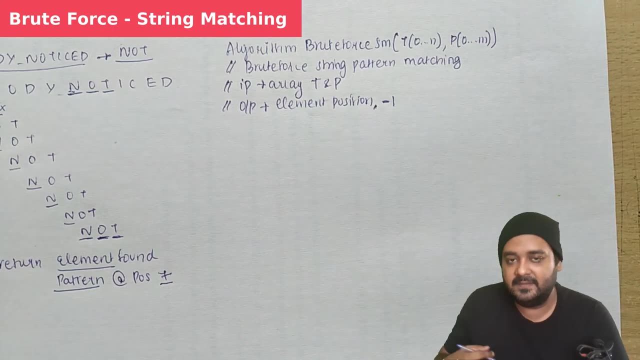 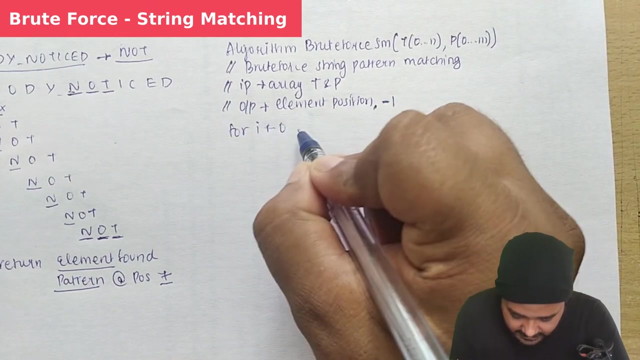 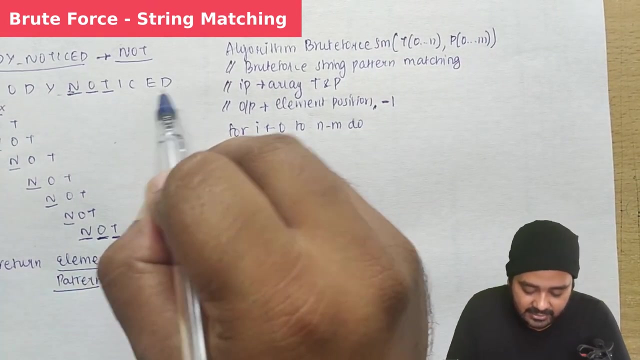 so if my element is present, it just returns the element position. if my element is not present, what it does? it just returns minus one. so minus one if the element is not present inside the list. okay, right, so for i is equals to z, zero, to n minus m. do so why am i mentioning n minus m means so, for example, here, there is no need. 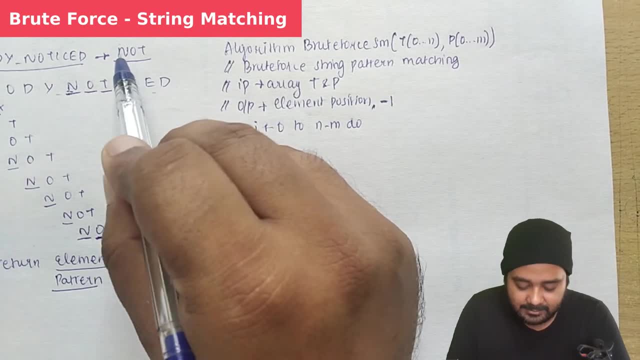 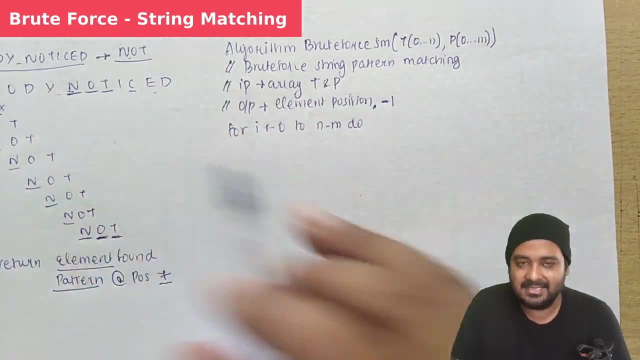 for you to check these last two elements. why? because is that the pattern is of length three, so here there are no elements further. so if we just stop with c, that's enough. why? because the last minus the length. so i'm just mentioning n minus m, right, okay, so i'm saying j is equals to 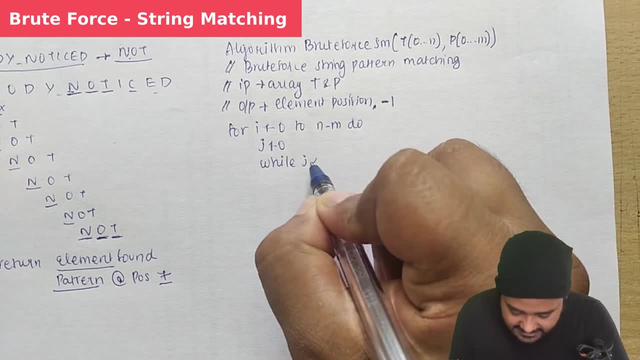 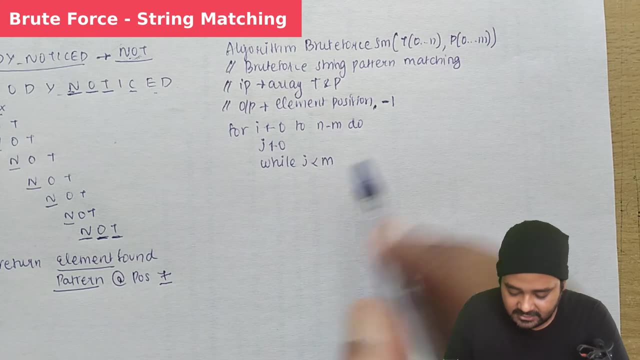 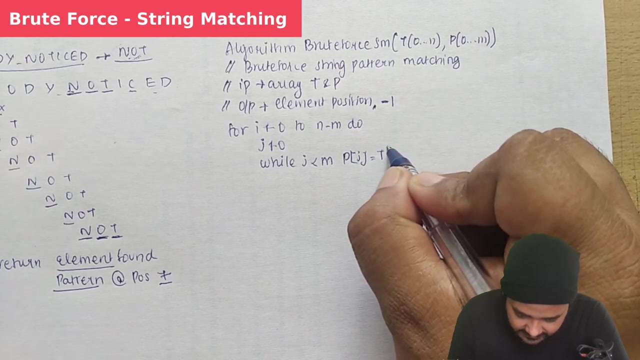 zero, right, so my, while j is less than equals to m. okay, so this is for this iteration. so the element to be found iteration: right, so for this iteration it is being mentioned. so p of j is equals to. okay, so text pattern: t of i plus j. do, right, so j is equals. 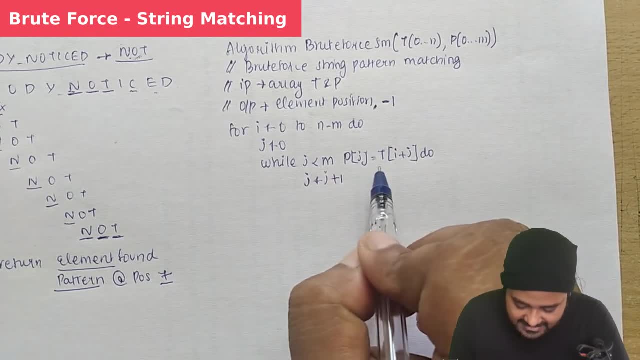 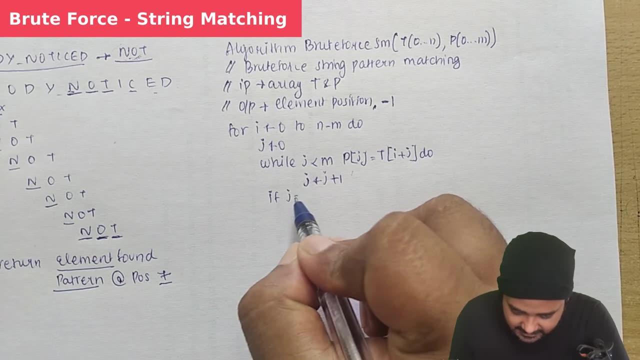 to j plus one. so we just keep on incrementing if it matches. so once it, if it is matched, we just have to move on it. so if it doesn't match, we just. there is no need for you to move. and then, if j is equals to m return. 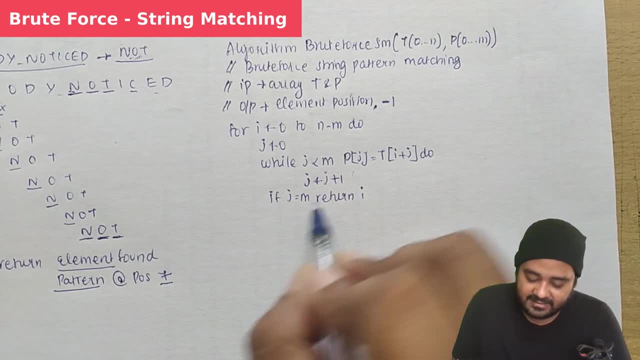 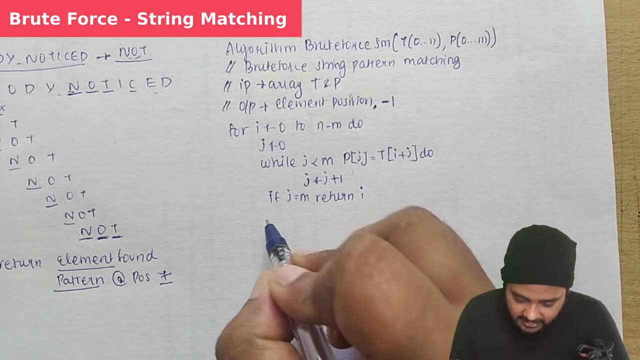 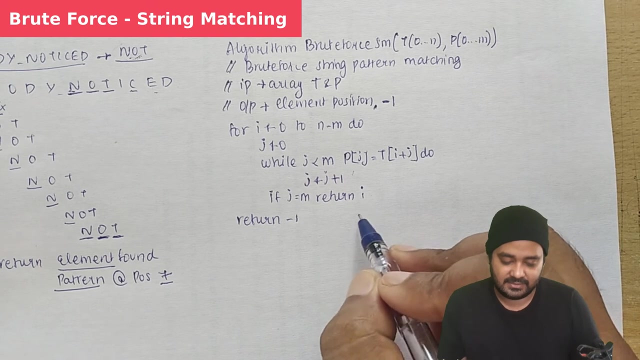 i right? so which means that if the element is being found, you just instruct your machine that you just have identified it and i'm just returning the position of it, or else what i do is i just return minus one. okay, so if the element is not found, it just returns minus one. so this is how. 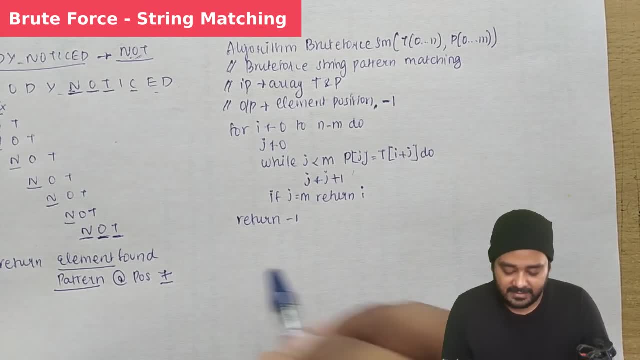 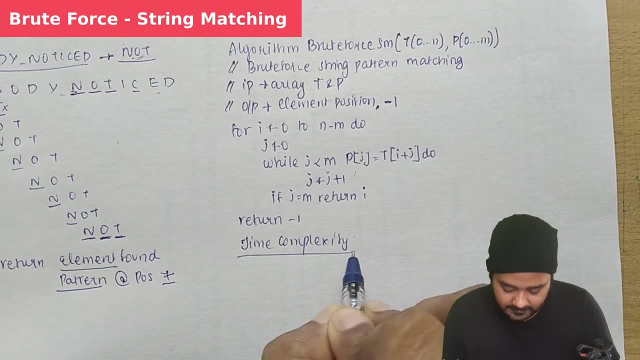 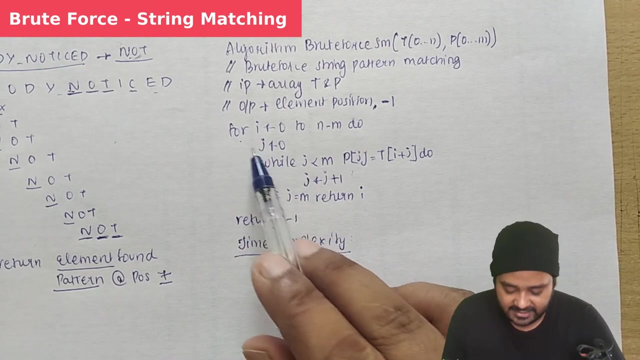 it works right, okay, so here, uh, the complexity. let's look at the time complexity of it. so time complexity, so looking at the time complexity of it. so generally, uh, we are having a couple of iterations, okay, so this iteration will range for n number of times, right? so we just know that this. 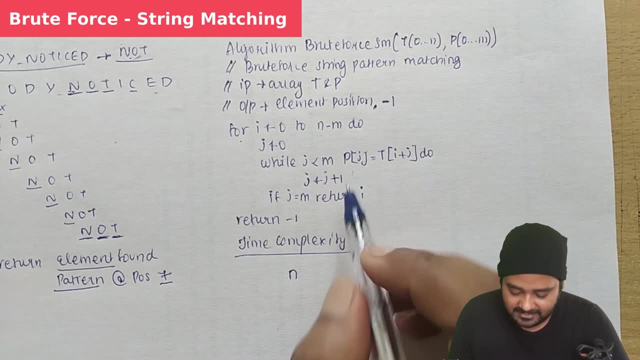 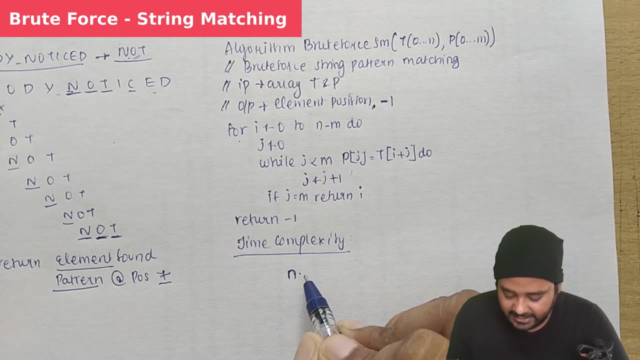 iteration will be ranging for n minus m number of times, and this iteration will be ranging to the maximum of m time, right? so, uh, right now, what we are going to do, we are just going to take n and then cross m, so maximum, uh, it will be leading. so, if it is going to be an worst case algorithm, so if it is a worst 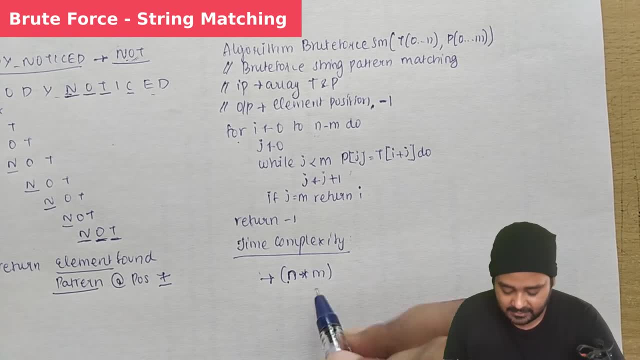 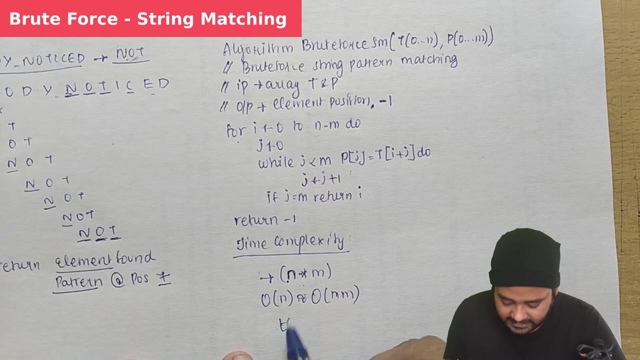 case algorithm, it just turns out to uh n star m. so uh for right now, i'm just mentioning my uh notation. so uh for n number of elements. the algorithms, uh tends to be uh, we go off uh n m right. so t of n. what is the time complexity? so t of time. complexity will n cross. m will be the. 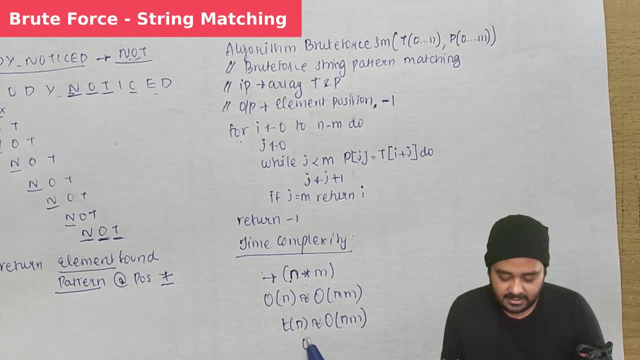 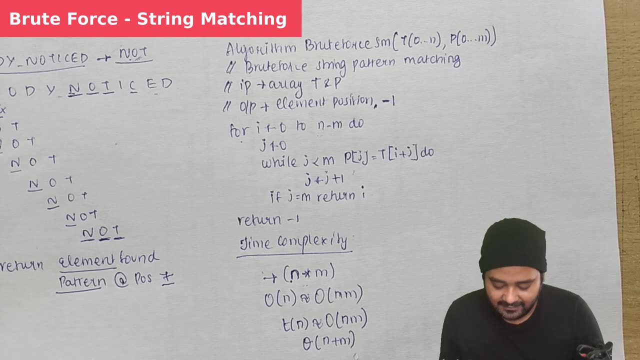 time complexity for the worst case algorithm. so if it is going to be uh, an average case, or theta notation, so it will be uh, something like n plus m number of terms for an average case. so this is how the string matching algorithm works, with the help of your brute force approach.